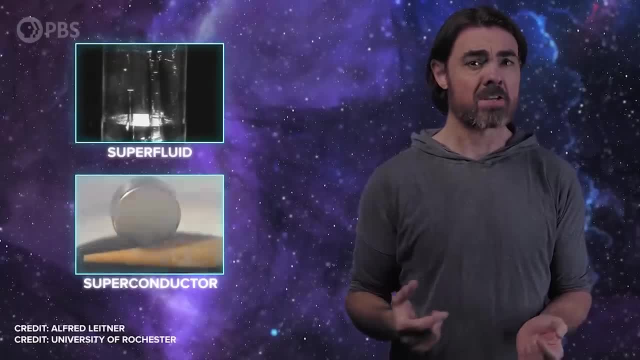 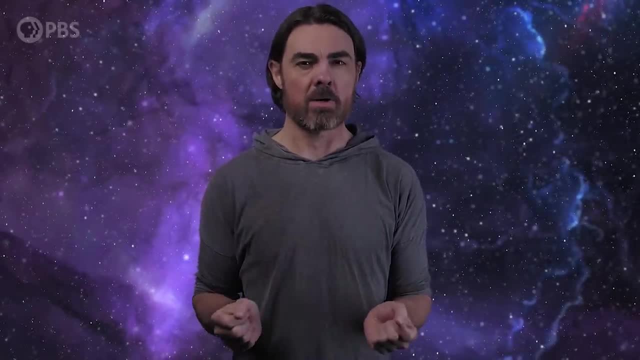 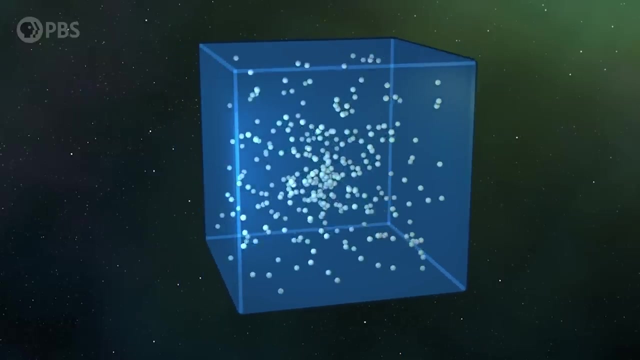 like superfluids and superconductors, and even allowed us to know whether a star will collapse into a black hole when it dies. To get started, let's try an experiment. We have a vacuum-filled room with no gravity and into it we blast a hundred rubber balls- Each ball. 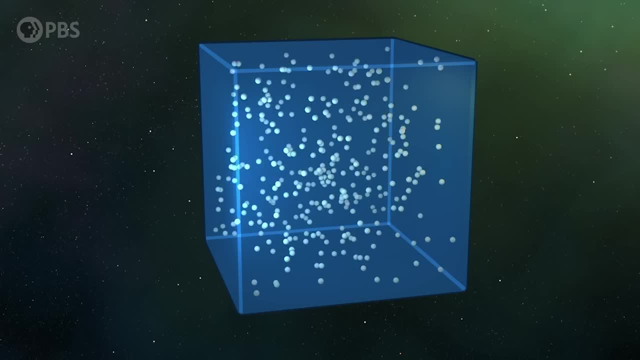 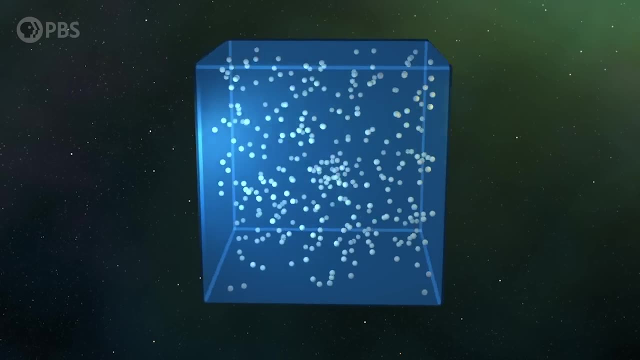 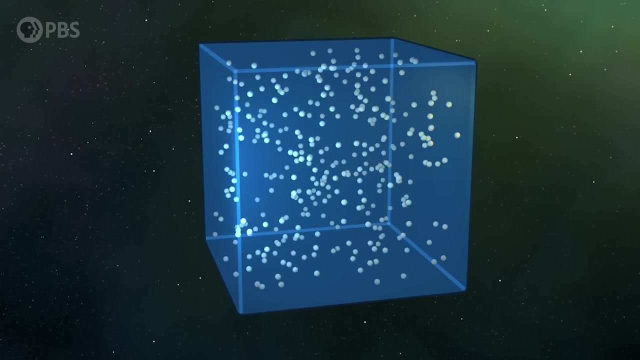 is small, perfectly bouncy, and is shot in at some random angle and speed. The balls are small enough that they never actually hit each other, but bounce off the walls without losing any energy. They're also moving fast enough that they quickly fill the room with a bouncy death storm. Let's 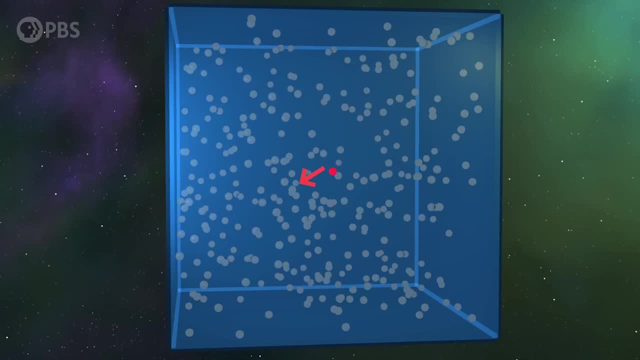 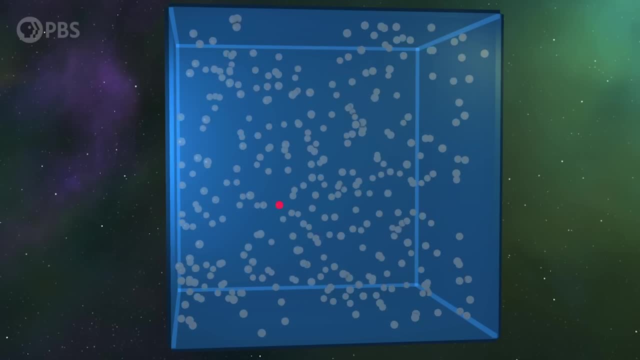 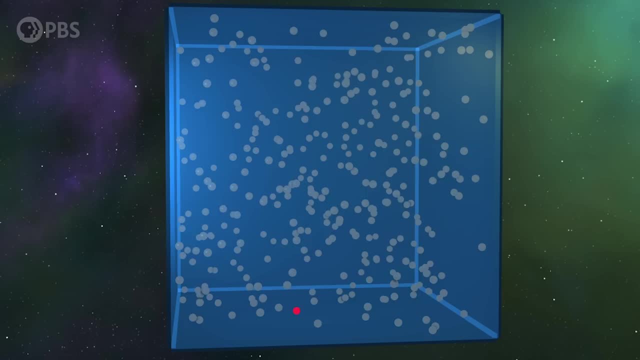 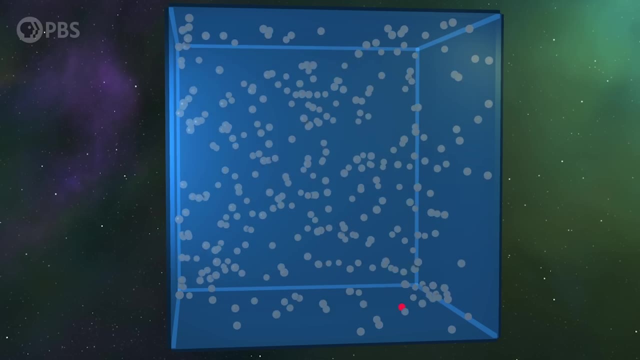 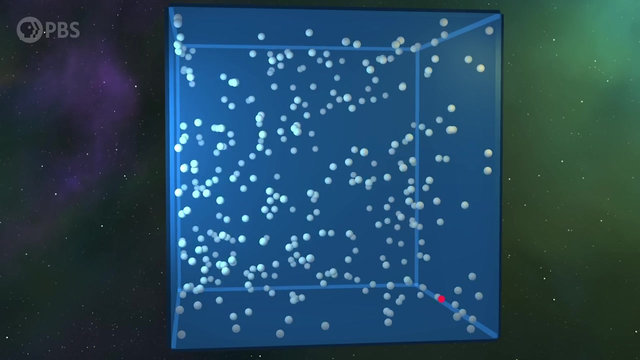 location will seem completely random. In fact, if we allow enough bounces, every possible location for that ball has effectively equal likelihood It could be anywhere in the room. But that also means that each configuration of locations for all a hundred balls is equally likely. 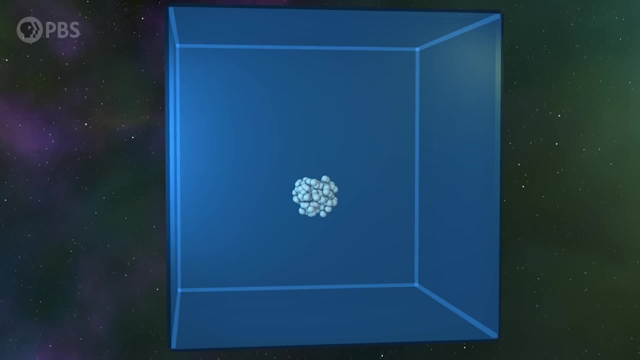 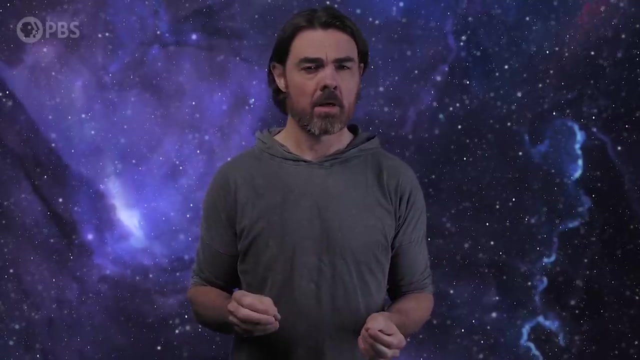 They could by chance all hit you in the head at the same time, Or or maybe they line up in a perfect lattice, or they could be haphazardly scattered through the room with no obvious pattern. That last one seems more natural, but actually any specific arrangement of balls is equally. 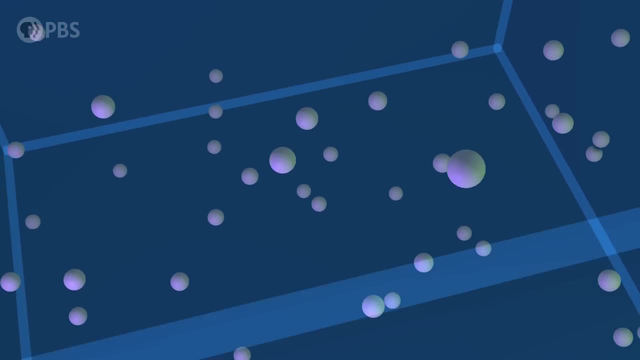 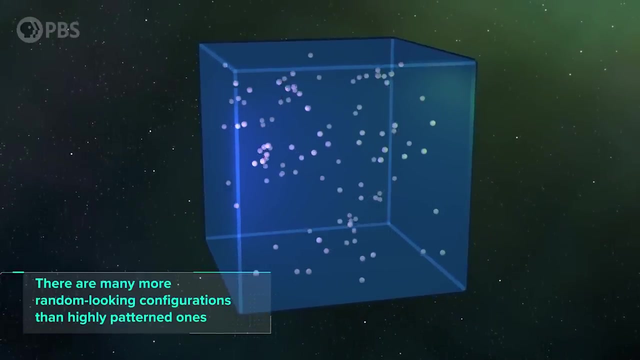 likely. The reason we're more likely to see a random-looking configuration is just that there are so many more room-filling random-looking configurations than there are highly patterned ones. To make this easier to see, let's divide the room into 10 boxes. 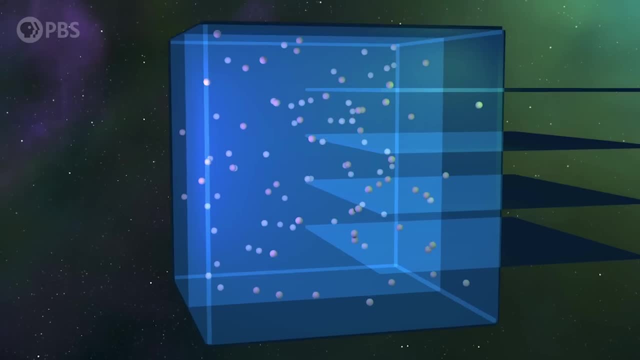 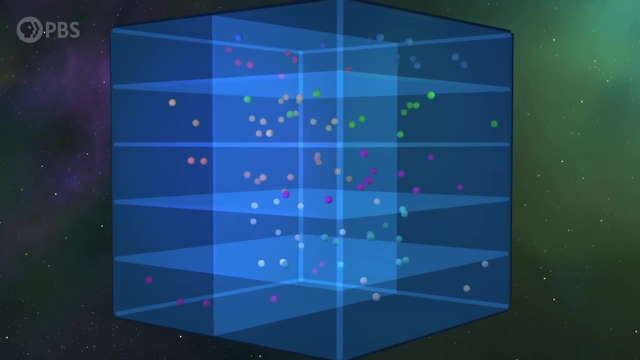 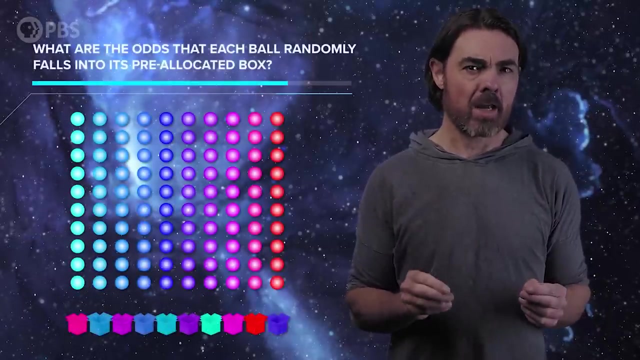 Spraying balls into the room is equivalent to randomly dropping them into those boxes. With 100 balls, we're much more likely to get a relatively smooth spread across the boxes versus them all landing in, say, the same box. But what if we label each ball and specify that each ball belongs to a specific box? 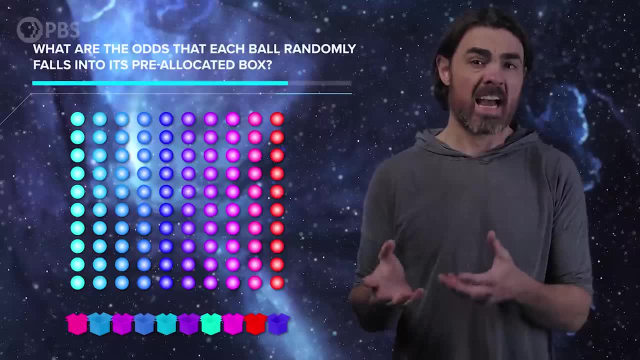 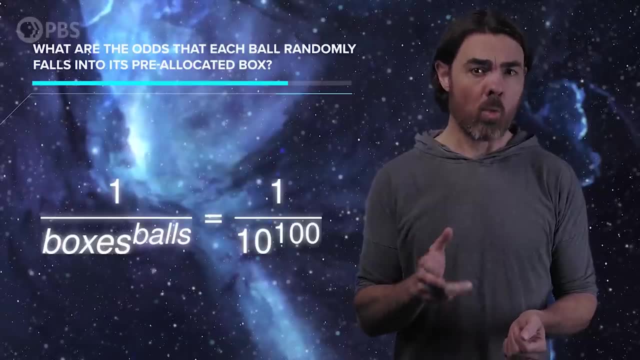 Now the chance of every single ball randomly falling into its pre-allocation is much lower. The probability of a box falling into a specific box is just as small as all the balls falling into the same box. Both have a probability of 1 over the number of boxes to the power of the number of balls. 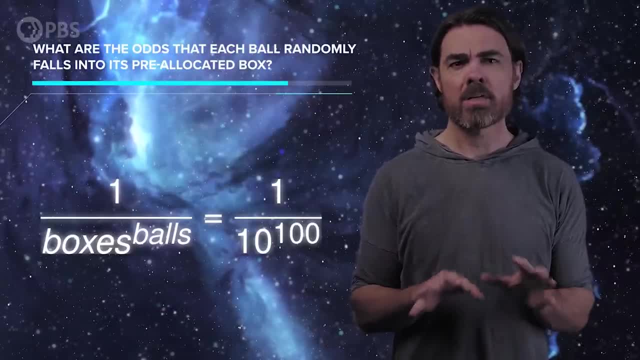 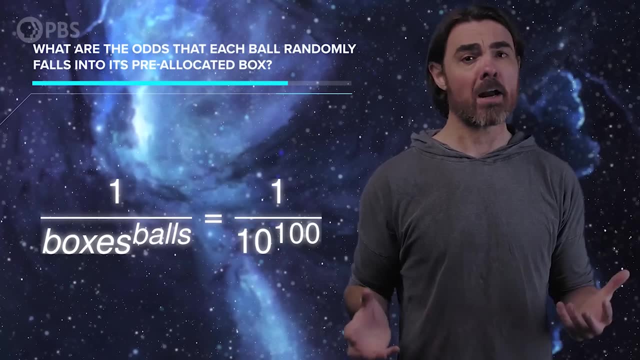 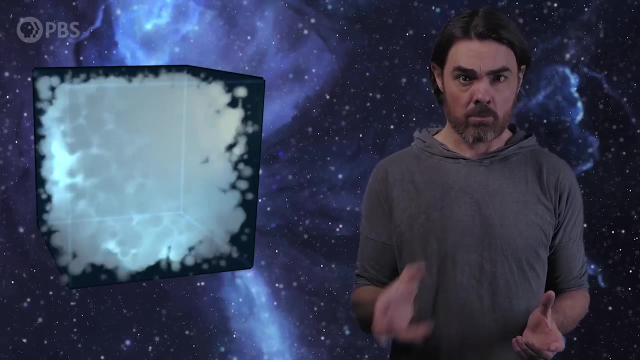 which is a probability so small that if you randomize the balls once every second, the Milky Way supermassive black hole will have evaporated before you get the balls in their right boxes. We can use this same idea to think about the state of molecules of air in the room, but 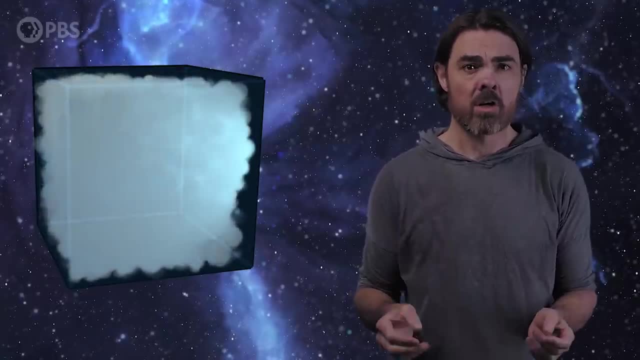 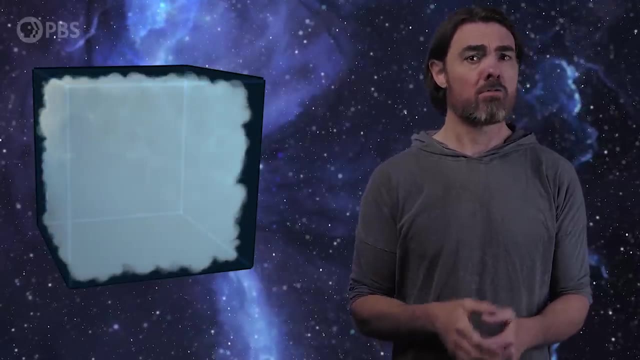 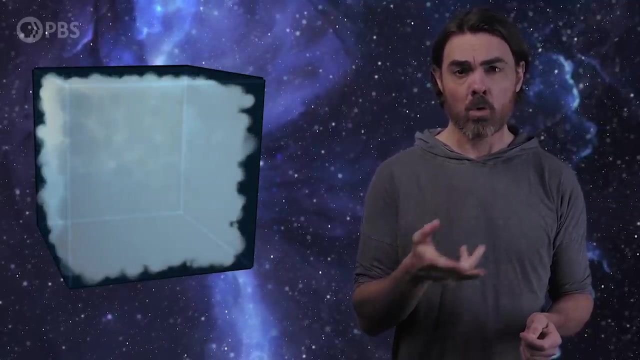 now we have 10 to the power of 27 particles instead of 100. So the chance of getting any one specific configuration is staggeringly unlikely. There are also vastly more configurations in which the air molecules are roughly evenly spread through the room than there are more ordered configurations. 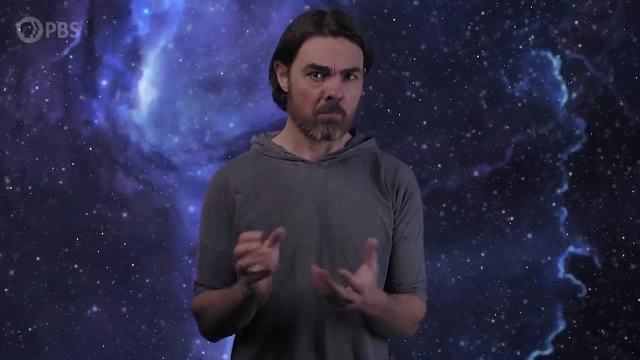 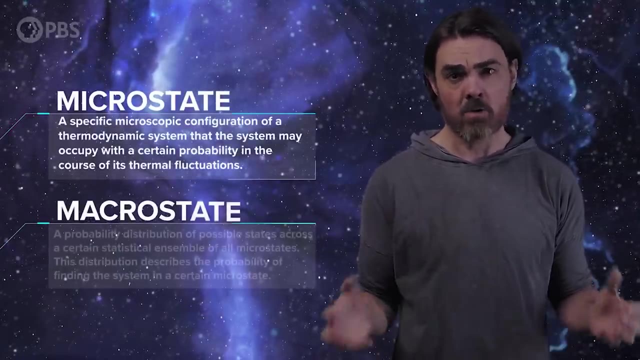 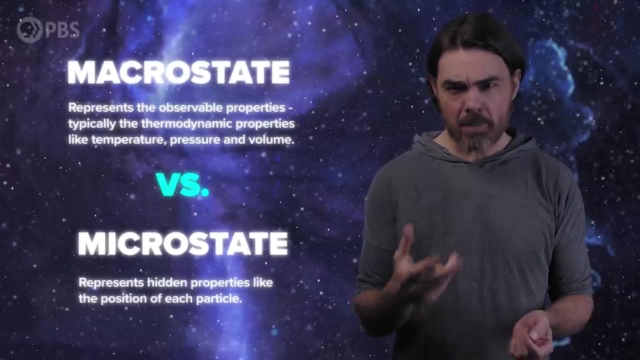 In statistical mechanics we call each specific configuration of balls or air molecules a microstate, While the general shape of the distribution, say, smoothly spreads, the mass of the air molecules, is a microstate. A macrostate represents the observable properties, typically the thermodynamic properties, like 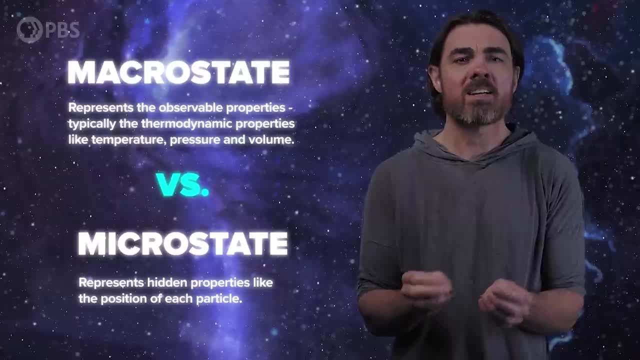 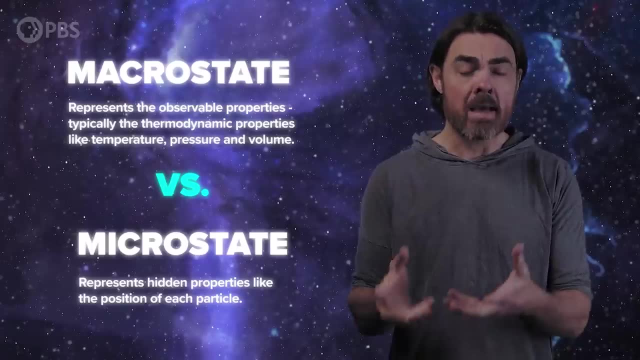 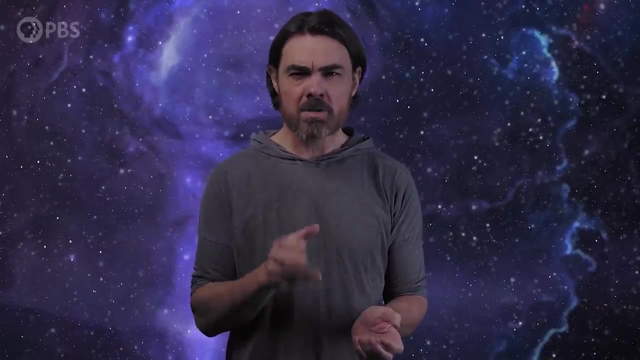 temperature, pressure and volume. Microstates represent hidden properties like the position of each particle, and each macrostate will correspond to many potential microstates. We almost always observe the world in the macrostate that has close to the maximum possible number of microstates. 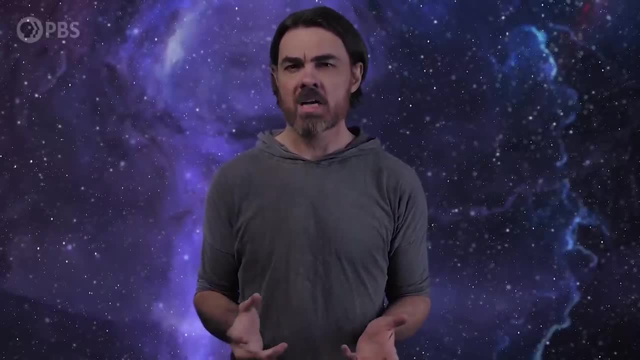 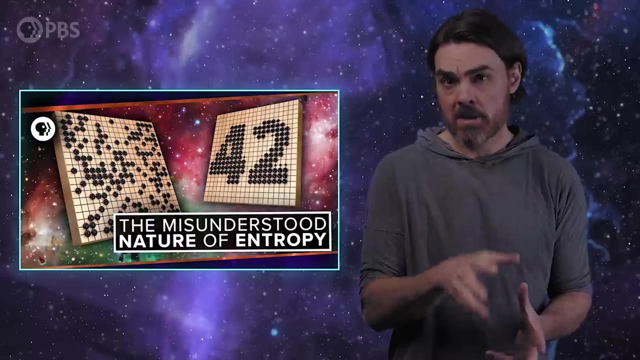 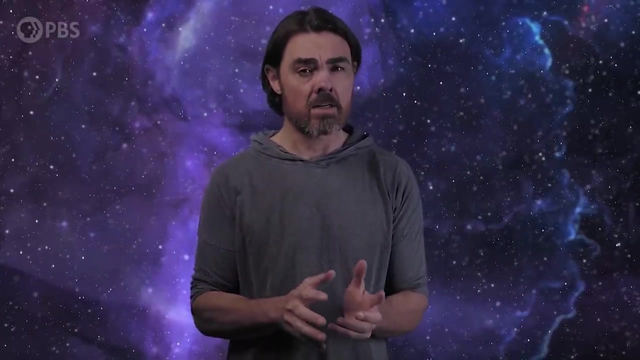 So what is a macrostate? We talked about this when we discussed entropy a while back. Entropy is a measure of how close your macrostate is to having maximum microstates, which corresponds to having the least amount of order. Systems always tend towards high entropy, but we can use these ideas about counting 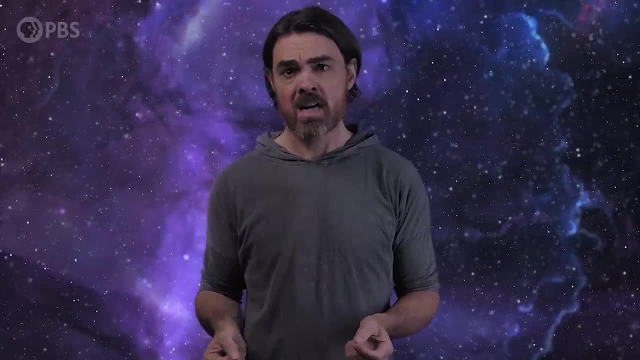 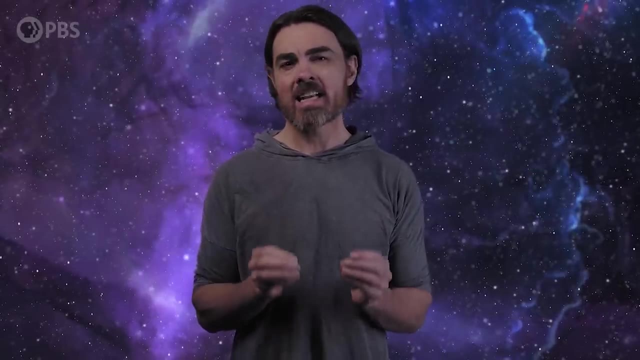 states to go a lot further than entropy in the laws of thermodynamics. To realize the full power of stat-mech, we need to stop thinking about macrostates as molecules are. Instead, we need to think about energy. Back to our bouncy balls. 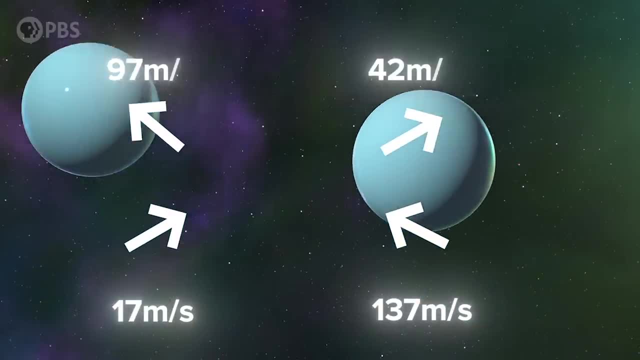 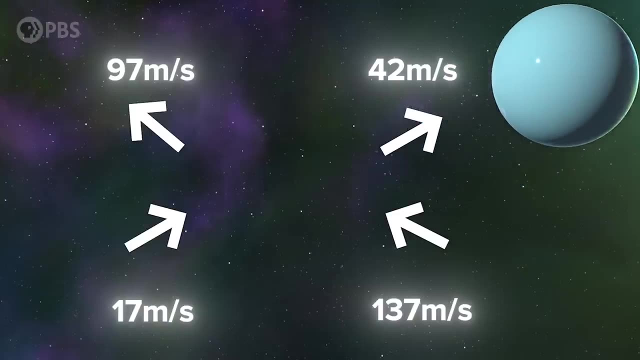 Let's imagine that they could also bounce off each other. As they move around the room, they change position and they also change velocity as they collide and so exchange energy with each other. We can think about their energy distribution in the same way that we thought about the. 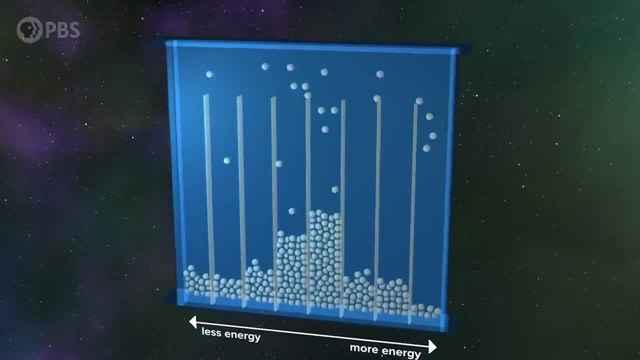 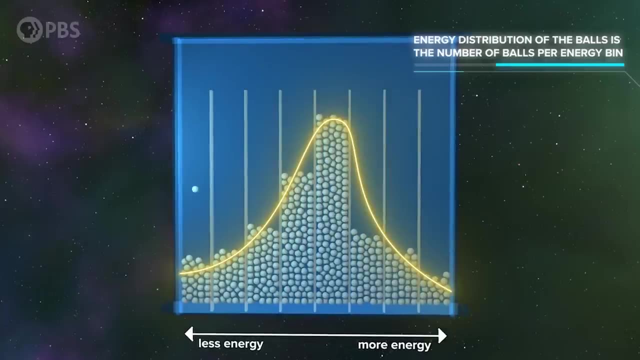 distribution of positions. Divide all possible energies the balls can have into a series of energy bins. If there are any energy bins for energy, then you can raise some energy. This is like this: The energy distribution of the balls is just the number of balls per energy bin. 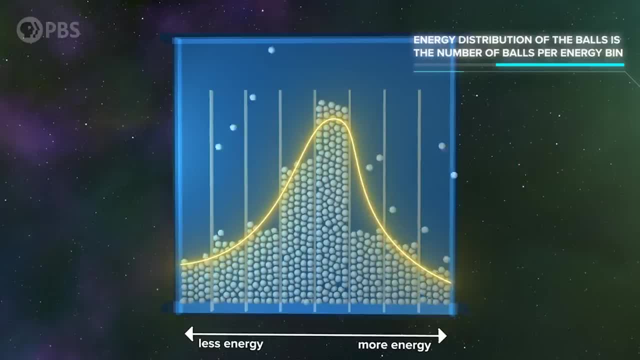 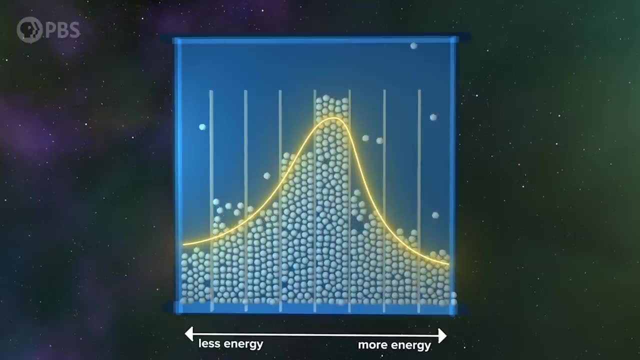 Just as with the positions, balls will move between energy bins as they interact And just as with position space, over time the system will explore all possible configurations of this energy space. Each specific distribution of energies is again a microstate, while the macrostate is. 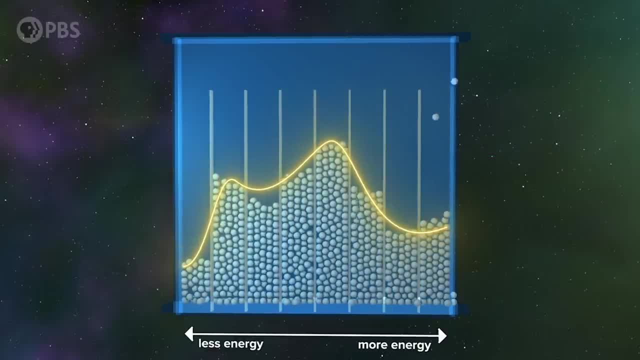 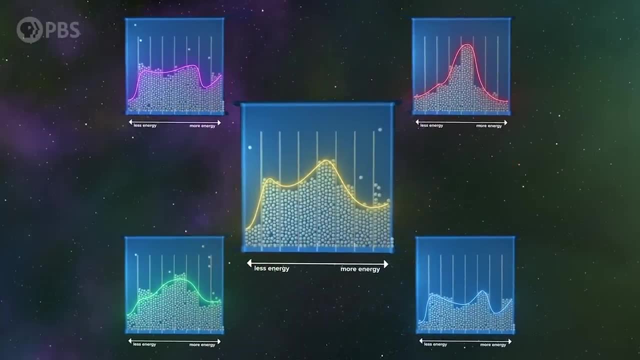 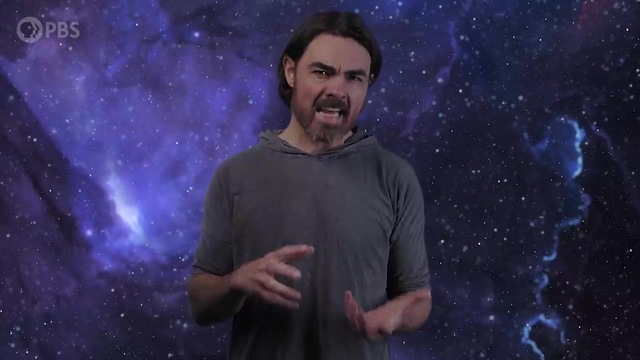 a particular shape of the overall energy distribution. For example, these are different macrostates And again, we're overwhelmingly likely to observe a macrostate and energy distribution that results from the largest number of microstates. The positions of the balls tended to become evenly distributed within the bounds of the 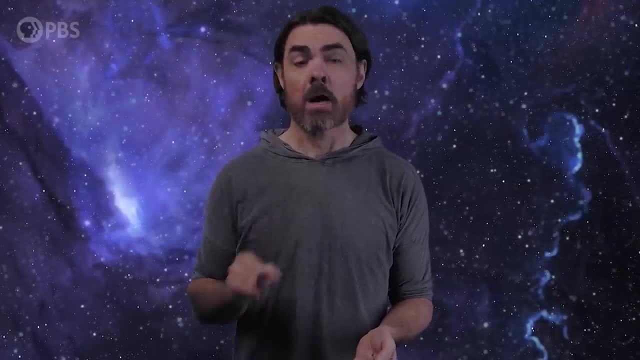 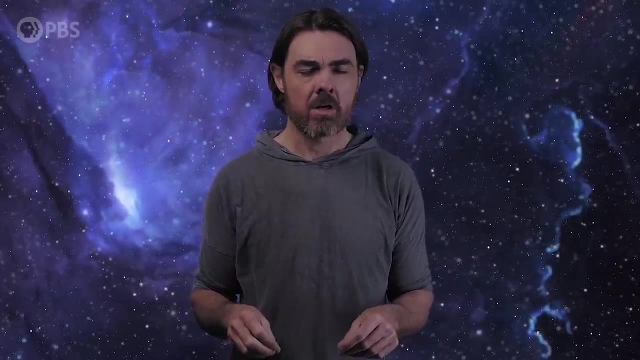 walls of the room. The energies of the balls are also constrained, but in a different way, And so the distribution of energies is not flat across all possible energies. The constraint is that energy is conserved. If one ball loses energy, another gains it. 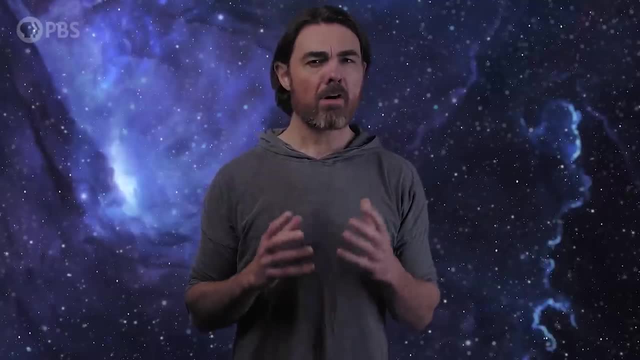 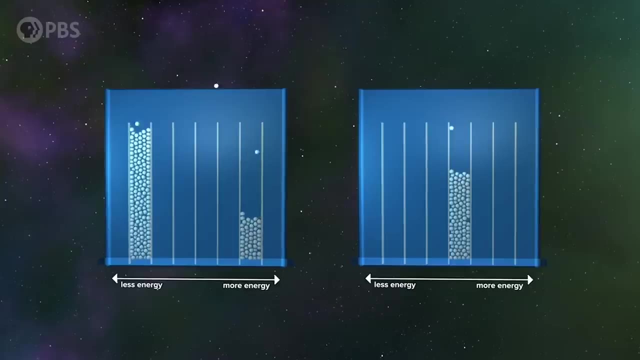 And the total energy of all balls always adds up to the same. There are various ways you can arrange out particles in their energy bins to get the same total energy, For example, splitting them between a high and a low energy bin or piling them all in. 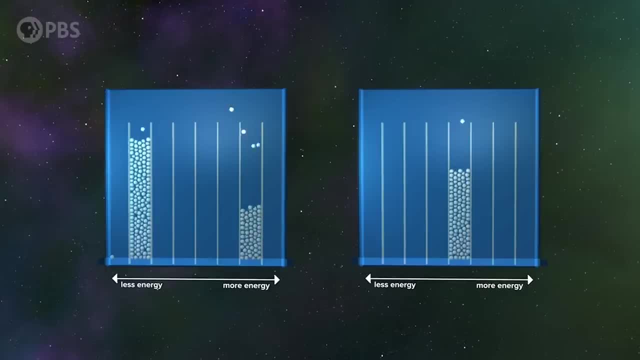 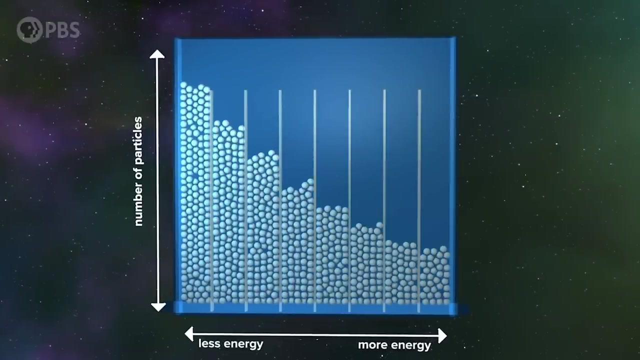 the bin corresponding to the average energy. Each of these distributions can be built with multiple different microstates just by swapping balls around within that basic spread, But there's a particular energy distribution that allows the most swapping, has the most microstates. It's something like this: 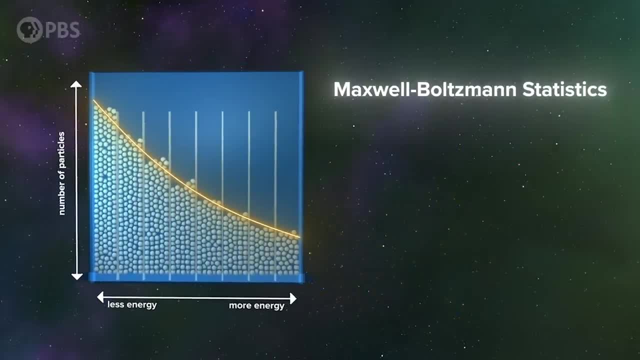 This is the energy distribution resulting from Maxwell-Boltzmann statistics, named for Ludwig Boltzmann and for James Clerk Maxwell. Mathematically it looks like this: It tells the number of particles in each energy bin and it depends on the temperature of. 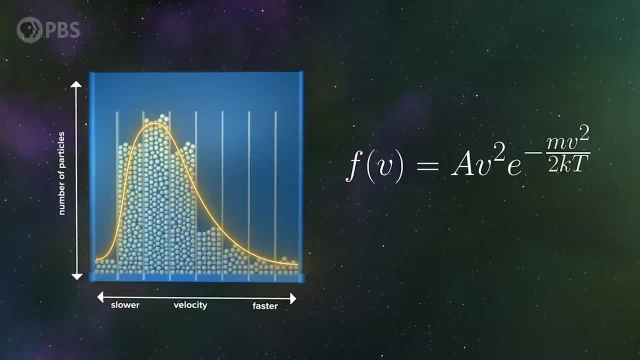 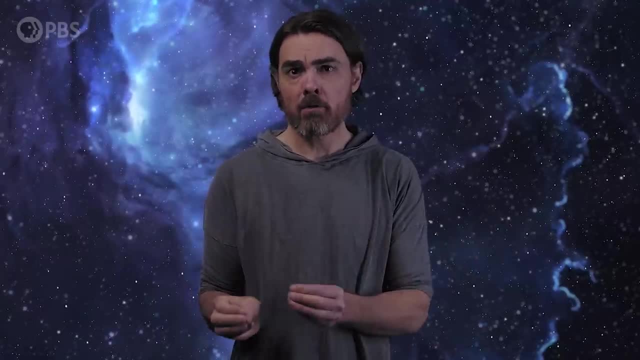 the material. From this we also get a distribution in particle velocities which is called the Maxwell-Boltzmann, The Maxwell-Boltzmann distribution, And all of this really just comes from counting the number of ways we can randomly put balls. 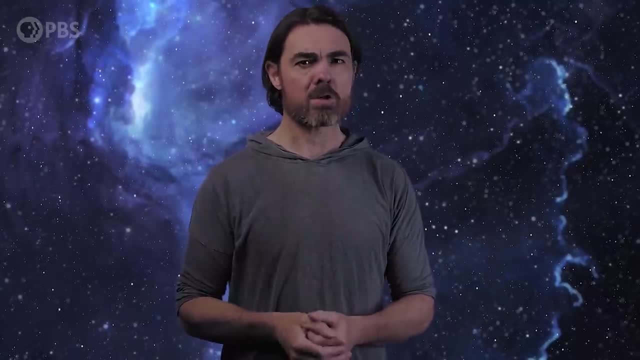 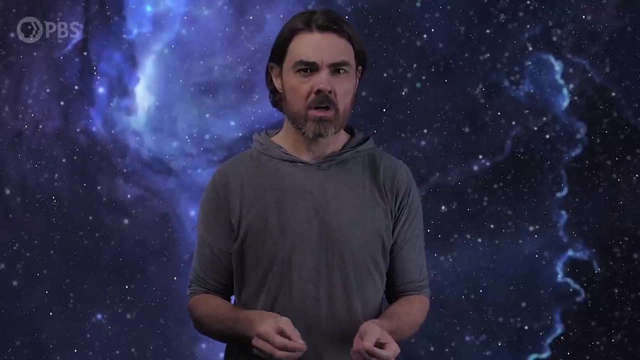 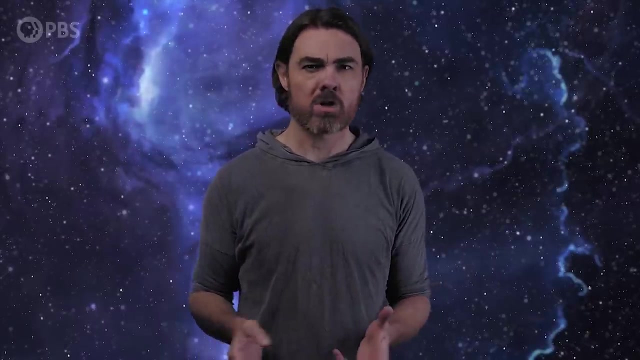 into different energy bins. The Maxwell-Boltzmann distribution represents maximum disorder or the highest entropy distribution of energies. just as high entropy is represented by particles filling the room in a random looking way. To give you some intuition about why it looks like this wonky bell curve rather than a flat. 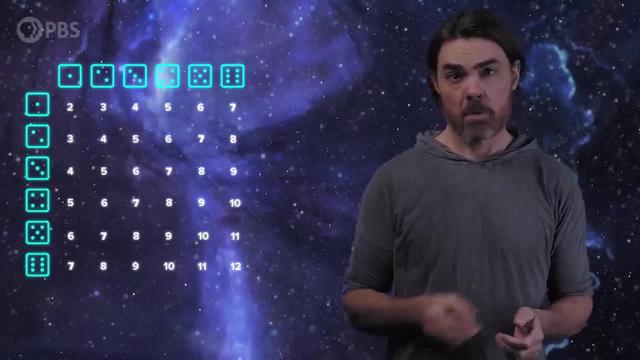 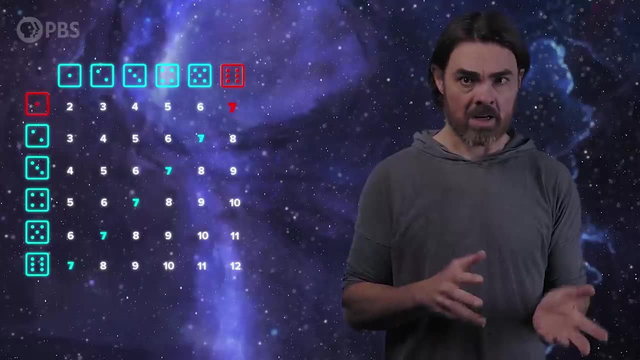 diamond. consider rolling our pair of dice. The most common number to roll is 7, and that's just because you can roll it in the most ways, Six ways in fact: 1 and 6, 2 and 5, 3 and 4, 4 and 3, 5 and 2,, 6 and 1.. Each of these number combinations is a microstate, all corresponding to the same macrostate of having rolled a 7.. The next most common macrostates are 6 and 8, with 5 ways to roll each, and the least common are 2 and 12.. 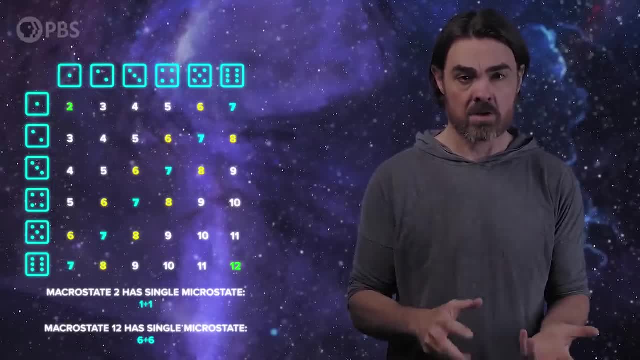 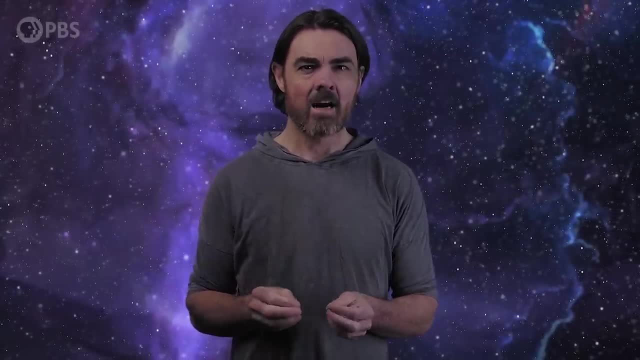 In other words, there's only a single microstate rolling two 1s or two 6s respectively. I did gloss over something pretty important in all of this. When I was counting energy states, I acted like it really matters which order you put. 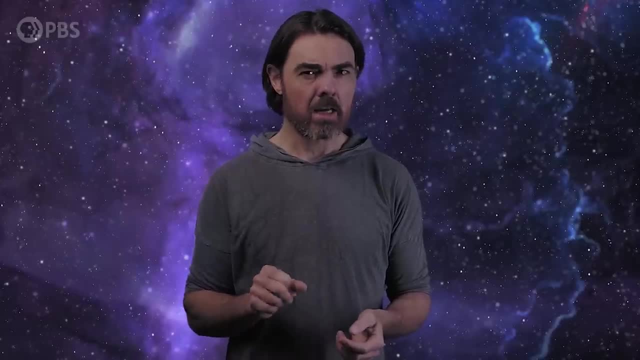 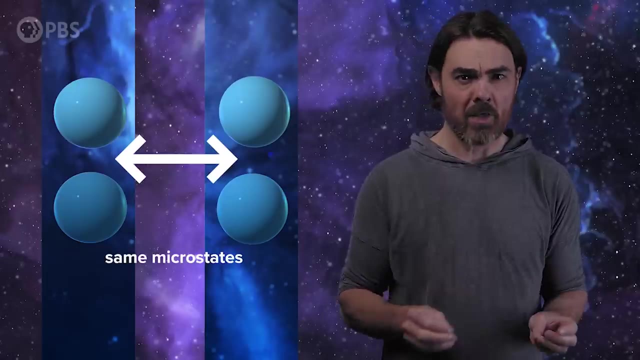 the balls into their energy bins. That's fine if the balls represent meaningfully distinct objects, but if the particles in question are truly indistinguishable from each other, then simply swapping two particles with each other shouldn't count as two different microstates. 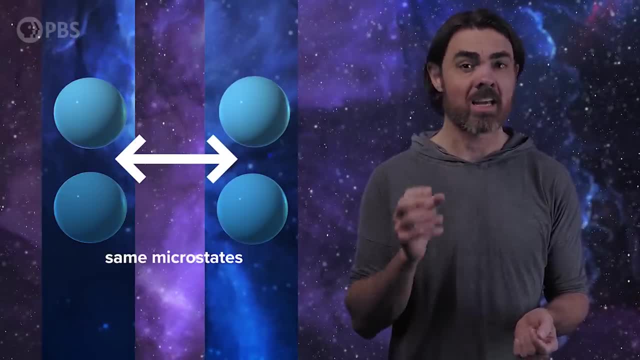 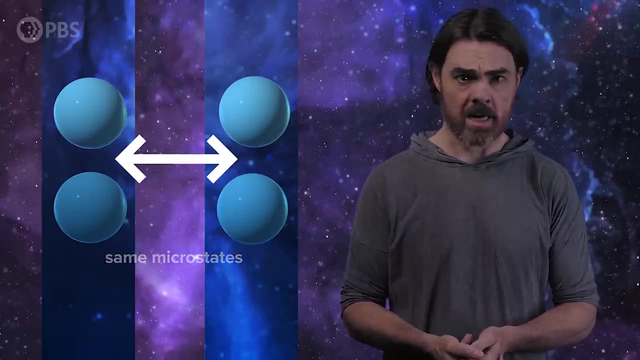 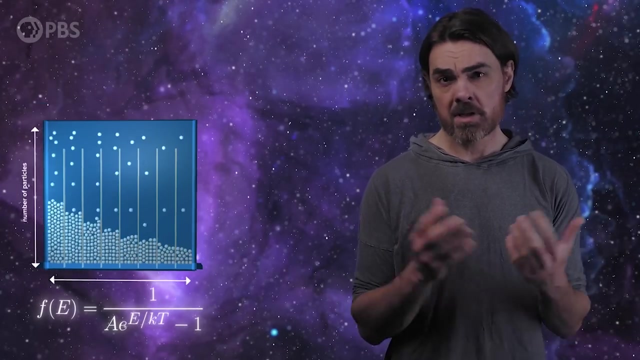 Changing the detailed spatial configuration counts, but not just mixing around the particle labels. So that means we have over-counted the states. When we count states correctly, this is the equation we get for the energy distribution. It was discovered by Satyendra Nath Bose, working with Albert Einstein, in 1925, and 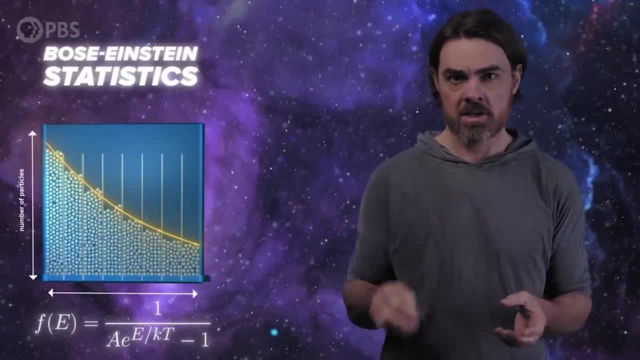 so we call this statistical behavior Bose-Einstein statistics. Any type of particle that behaves in a certain way is called Bose-Einstein statistics. This is the equation we get for the energy distribution. Any type of particle that behaves in a certain way is called Bose-Einstein statistics. 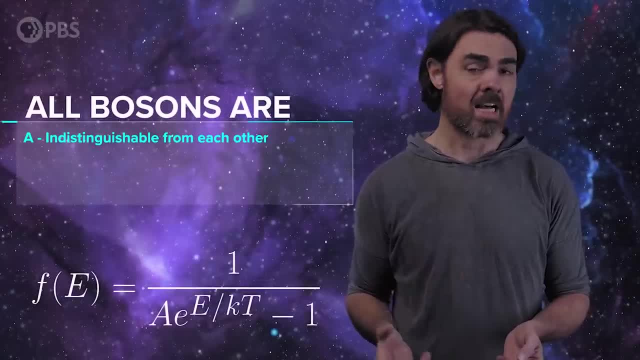 Any type of particle that behaves in a certain way is called Bose-Einstein statistics. This is the only California cerc glued to an object called a Bose-Einstein data set, And it almost alwaysbreviets only the whole wave into operator. Awkward vision. 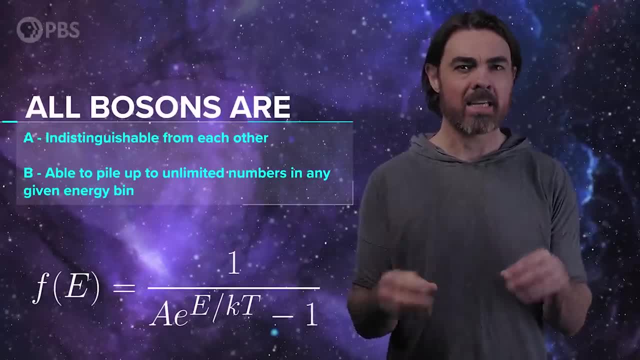 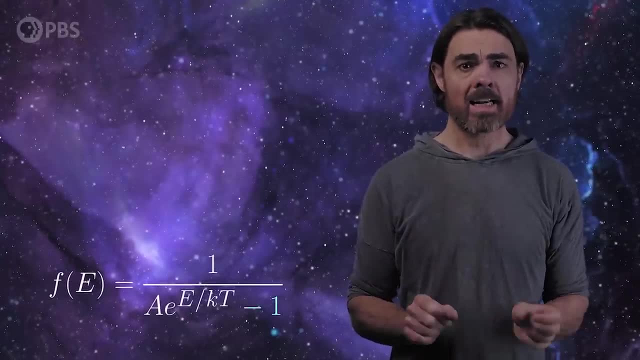 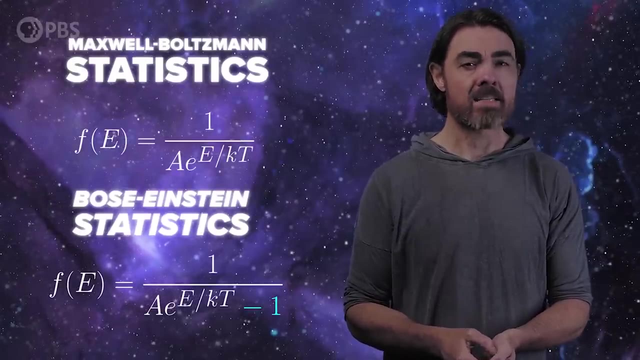 The question is: why is it even possible that any third or even multipleètres exist all at once? when equating a minimum sine wave to some count, It's all possible, but how doth that? Let's not make all the deductions, But a hundred beginners can handle that question absolutely easily. 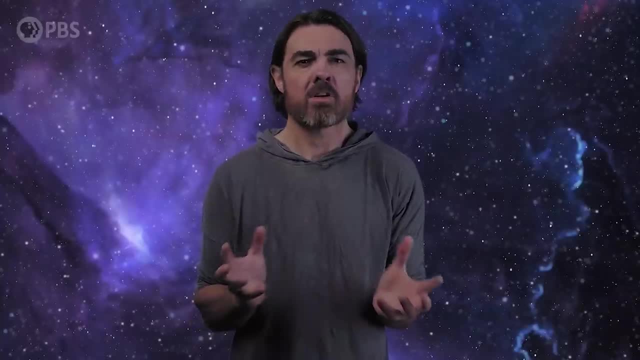 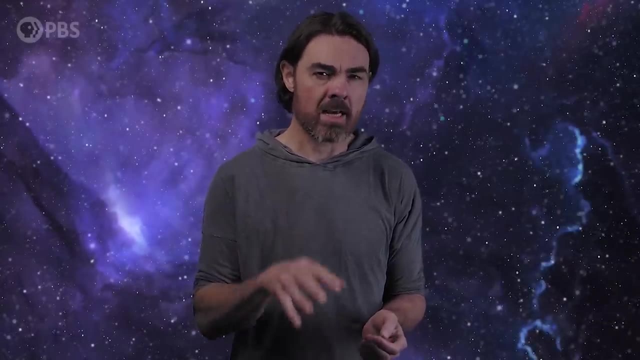 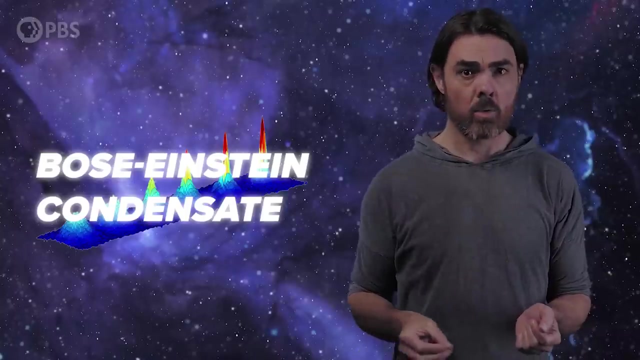 But how about using this exact equation- all right, particles per energy bin- making it possible to cram way more particles in the lowest energy states? This results in an entirely new state of matter: the Bose-Einstein condensate, which manifests as superconductivity, superfluidity and various other weird behaviors, depending on the material. 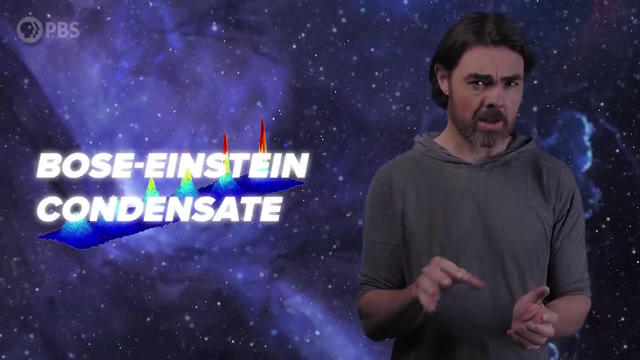 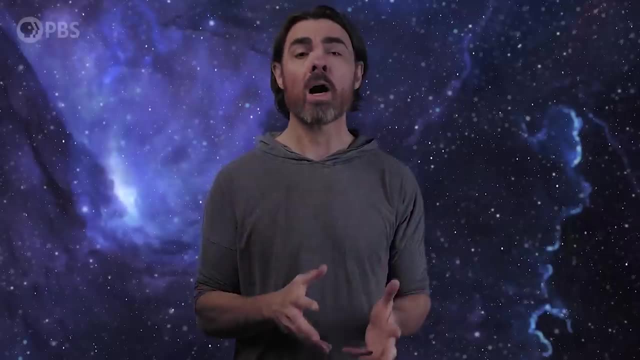 We're going to come back to Bose-Einstein condensates in more detail another time. For now, we're going to wrap up with one last way of counting states that leads to wildly different behavior. For Bose-Einstein and Maxwell-Boltzmann statistics, there's no limit to the number of particles. 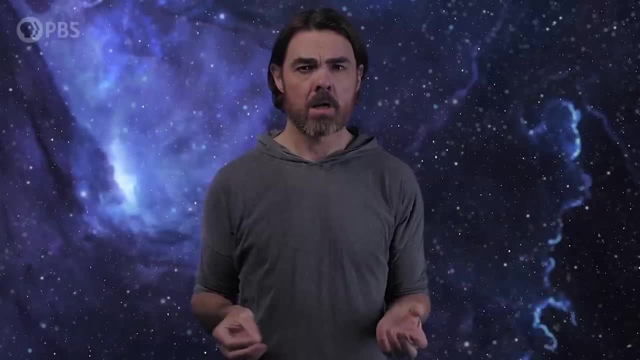 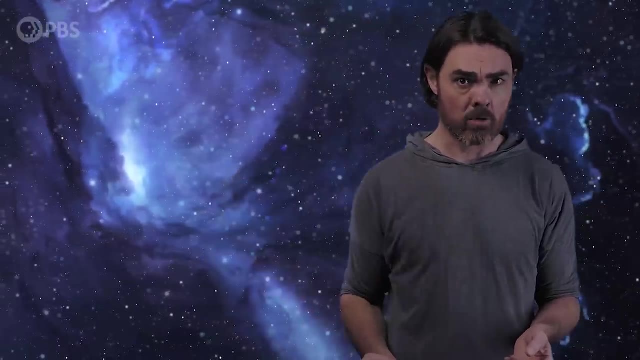 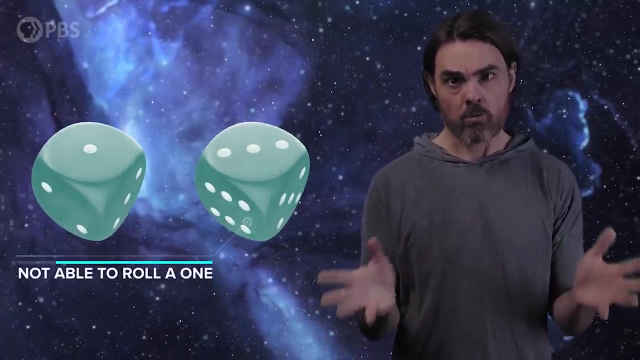 per energy bin, but that's not true of all particle types. Some particles refuse to share their energy bin, so that each energy state can only be occupied by a single particle. It would be as though rolling a 1 on one die meant that the other die could not also roll. 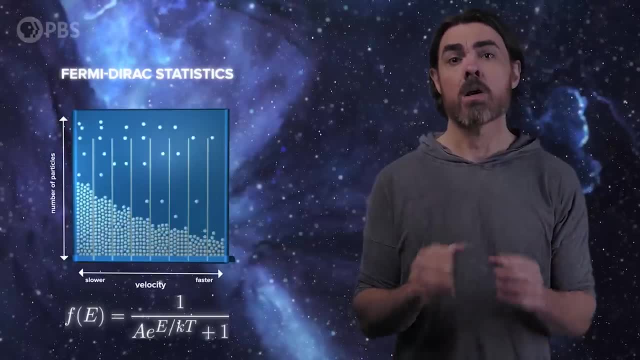 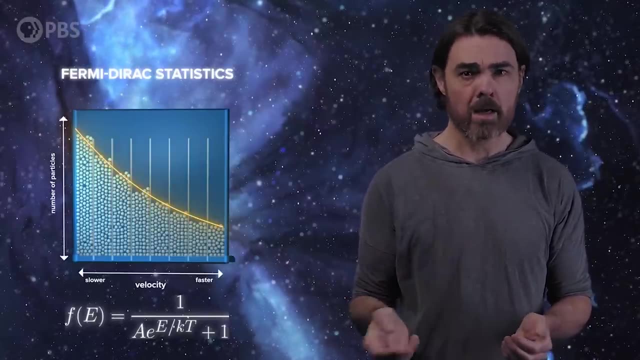 a 1. You need to count the possible states of such particles very differently, and the result is Fermi-Dirac statistics, named for Enrico Fermi and Paul Dirac, two of the founders of quantum theory. Particles obeying these statistics are called fermions. 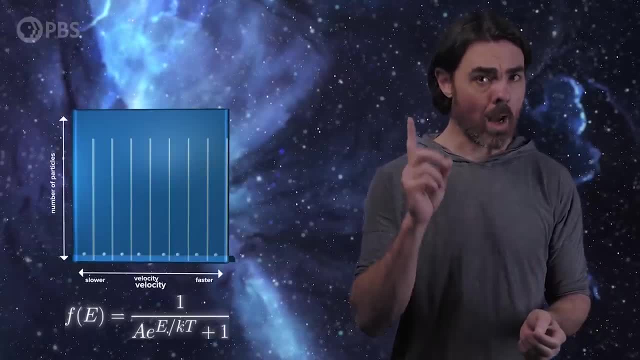 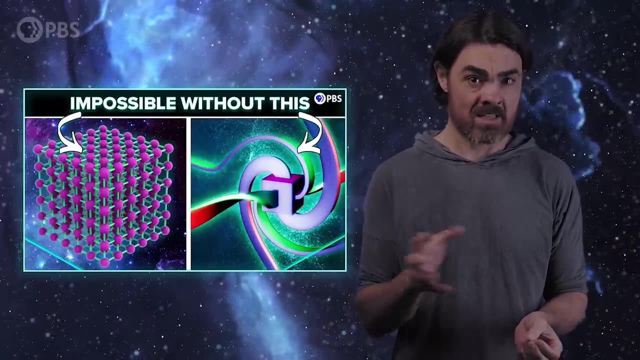 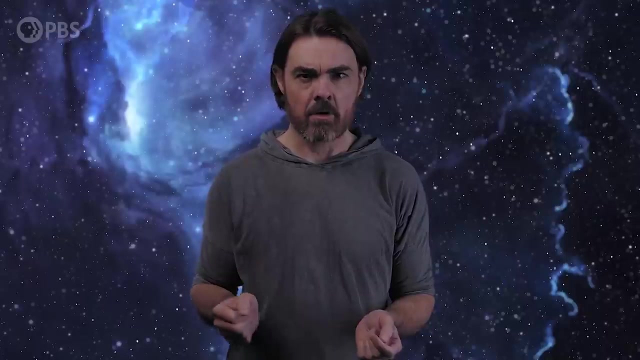 Fermions are indistinguishable and they are restricted to 1 per energy bin. We talked about why exactly some particles should suffer this restriction in our episode on spin statistics, But, in short, Particles with a quantum spin value that's half integer are forbidden. 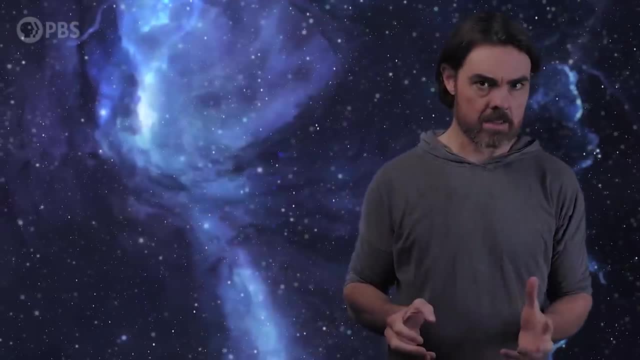 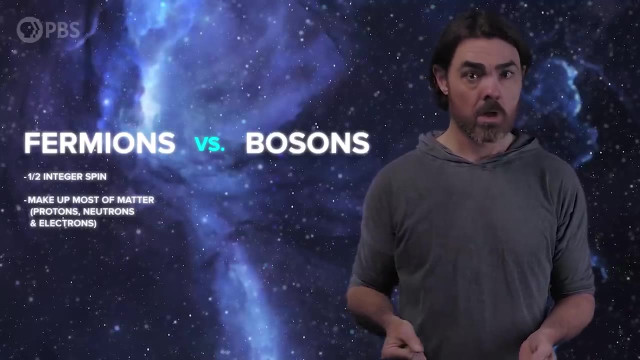 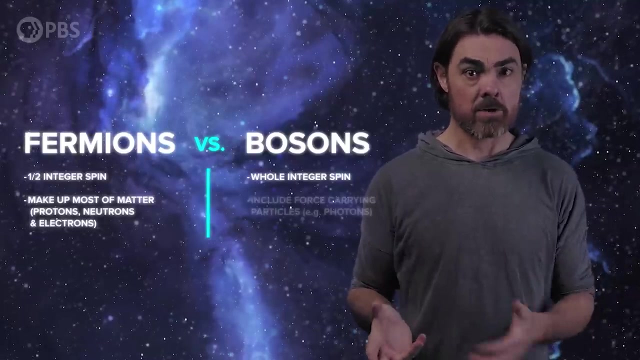 from overlapping because quantum mechanics These are fermions and include the particles that make up most of matter: electrons, protons and neutrons. Particles with integer spin are bosons and include the force-carrying particles like photons. But you can also make bosons out of combinations of spin-half fermions, for example the helium-4. 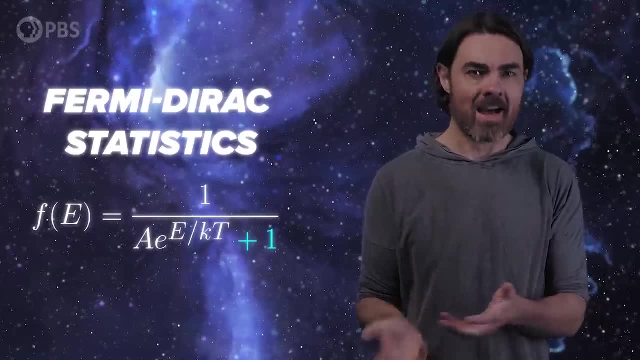 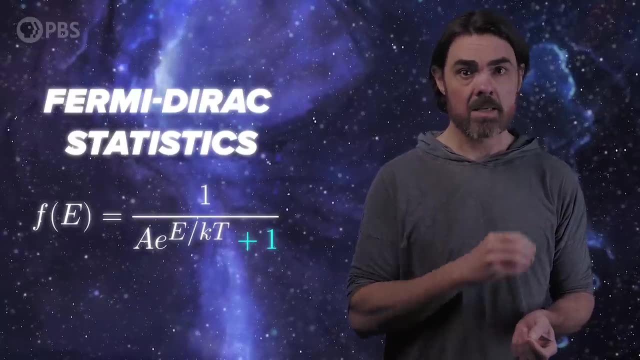 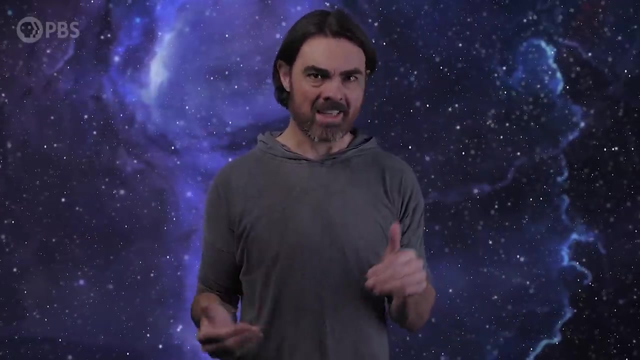 atom Fermi-Dirac statistics look similar to our other statistics types, but now the minus one from Bose-Einstein becomes a plus one Again. this makes little difference for high temperatures, but at low temperatures things get weird, Because fermions can't all fall into the single lowest energy state. they instead fill. 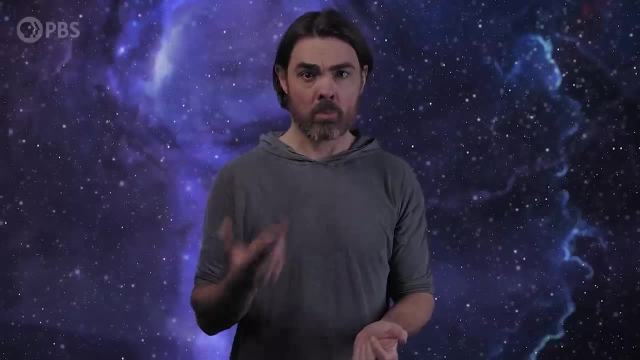 up all of the available low-energy states with one particle per state. This leads to nice things, like the fact that electrons in atoms can only have one particle per state. This leads to nice things, like the fact that electrons in atoms can have only one particle per state. This leads to nice things like the fact that electrons in atoms can have only one particle per state. This leads to nice things like the fact that electrons in atoms can only have one particle per state. This leads to nice things like the fact that electrons in atoms can have only one particle. 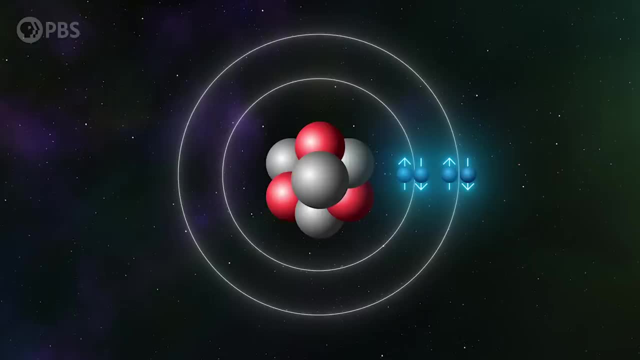 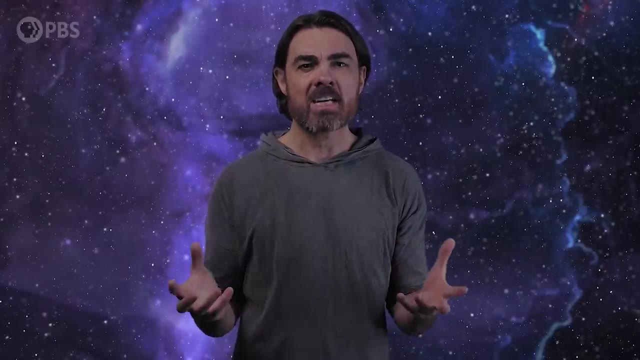 per state. Either way, the seven electron spin allows up to two electrons to be distings from each other with opposite-pointing spins, But the result is that atoms are much larger that they would be if electrons were bosons With opportunities of palabry, not of clinic. 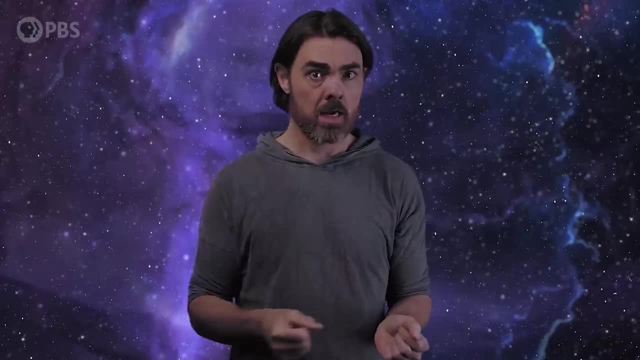 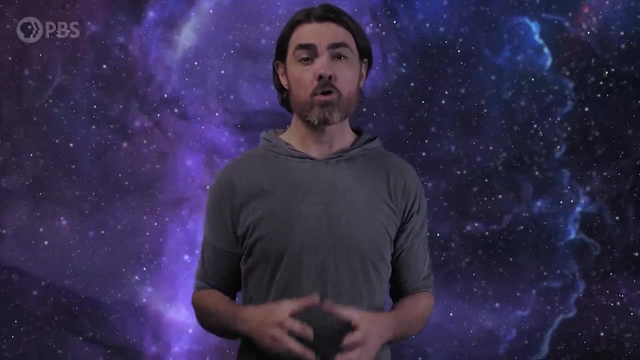 Hence we spin electrons per energy with one particle per state, And this is why we have chemistry and structure in this universe. The strange behaviour of Fermi-Dirac statistics also leads to some of the weirdest objects in the universe: White dwarves or neutron stars. 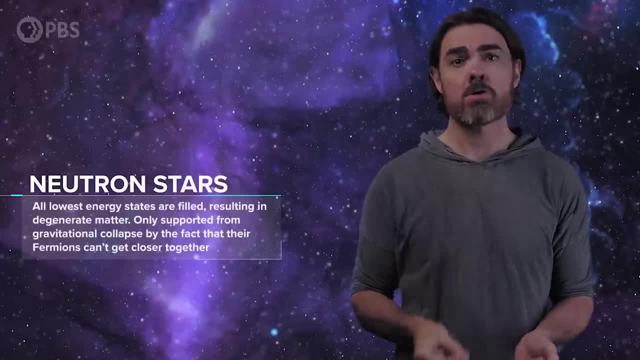 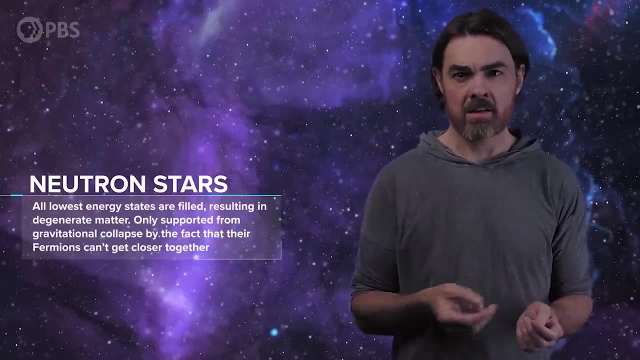 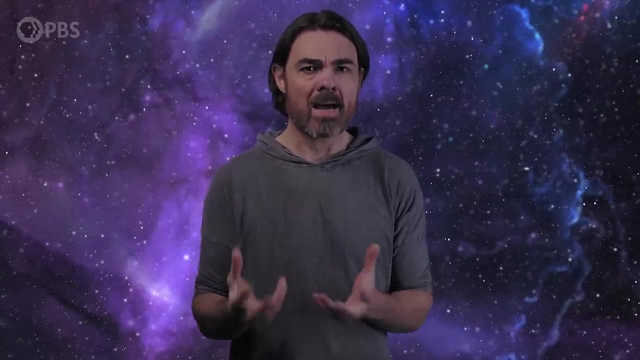 where all of the lowest energy states are filled, resulting in what we call degenerate matter. These things are only supported from gravitational collapse by the fact that their fermions can't get any closer together, and it was by using Fermi direct statistics that we figured out how massive a star needed to be in. 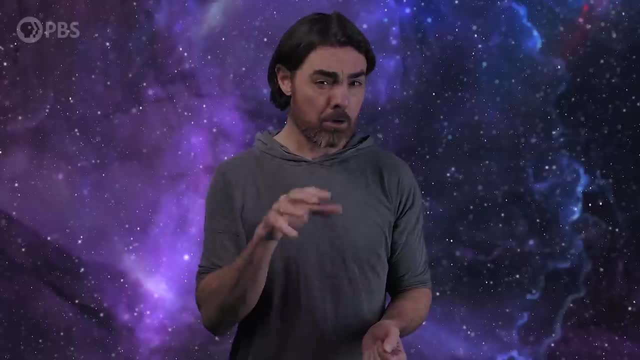 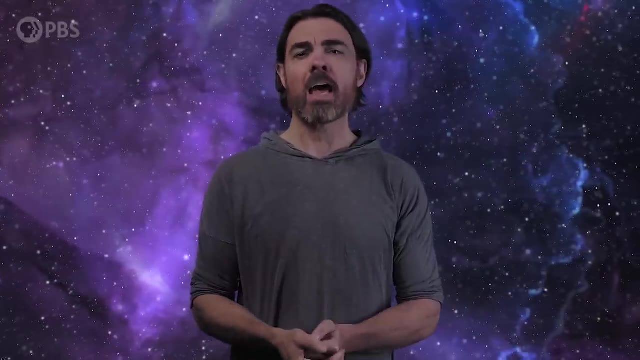 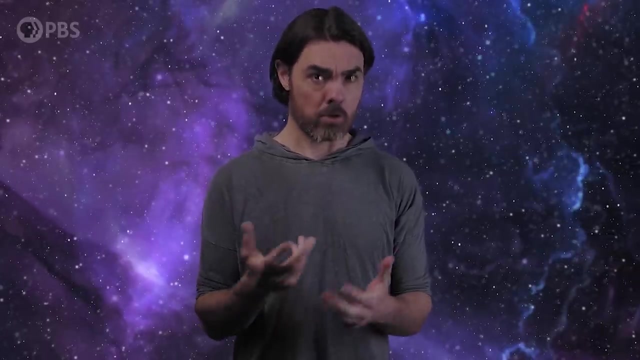 order to collapse through the white dwarf phase and through the neutron star phase into a black hole. Of course, we've also talked about that previously. Okay, so that's all I have to say for now about statistical mechanics. It's all about counting. We perceive the crude properties of the universe and its 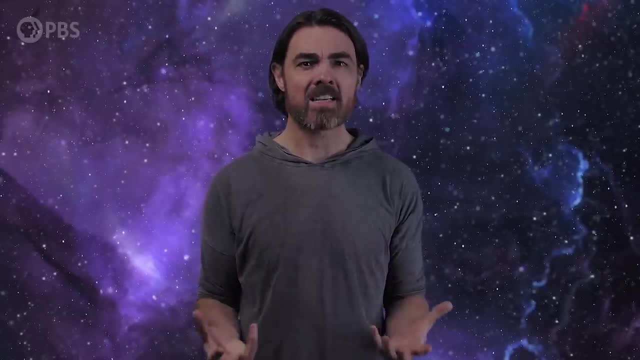 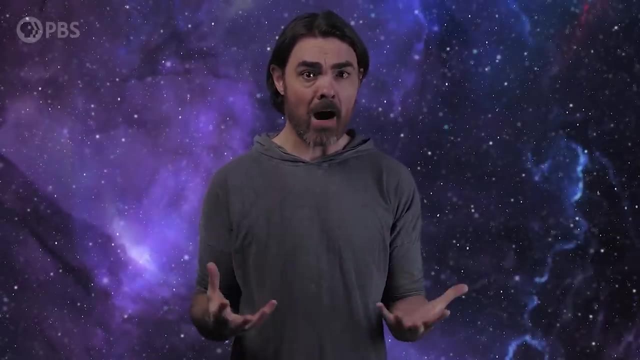 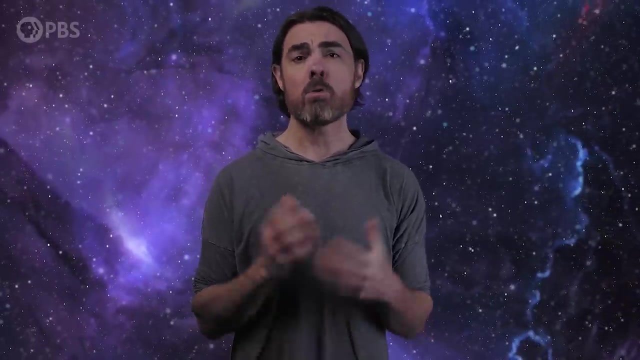 details are hidden from our view, but simply by counting the different hidden ways by which those crude observable properties may have come about, we gain great power in predicting how these observables will behave. By mastering the game of cosmic craps, we come to a new understanding of the origin of the 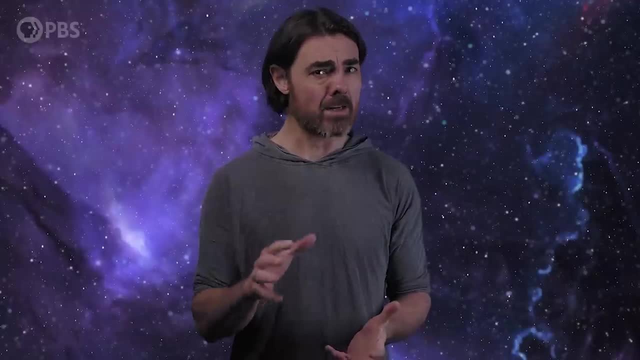 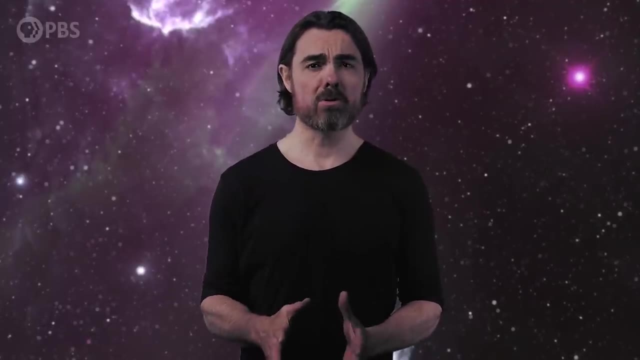 physical universe And that's what we're going to talk about in the next episode of Space Time. Before we go, I want to thank everyone who supports us on Patreon and to let you know that I did a live stream comment response for the last six episodes.